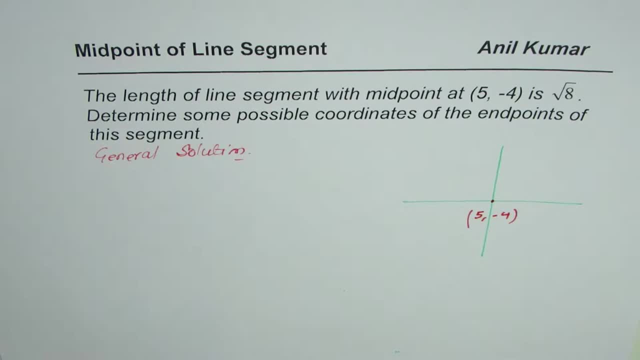 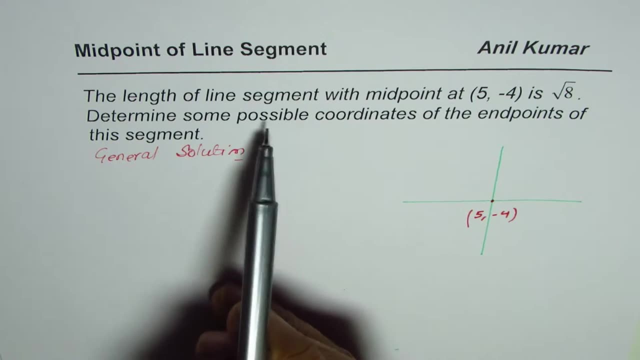 So that is the whole idea. to make it more interesting, And you will notice that the endpoints are some possible coordinates. So some possible coordinates. I'll give you one set of coordinates. You can find others right. So that's the whole idea, Okay, So. 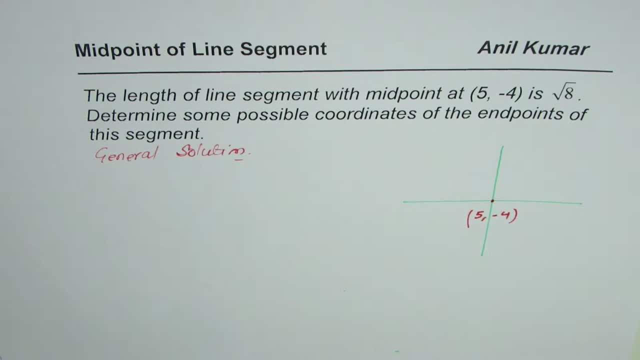 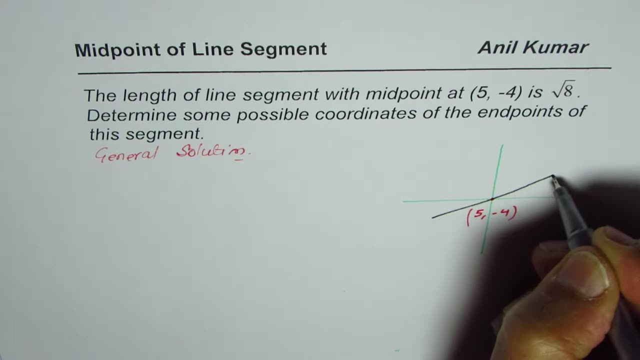 what we will consider is just let me sketch a general line here. Let us say: this is our line, going through the point 5 minus 4, and these are my endpoints, right? So I am saying these endpoints are A and B, right. 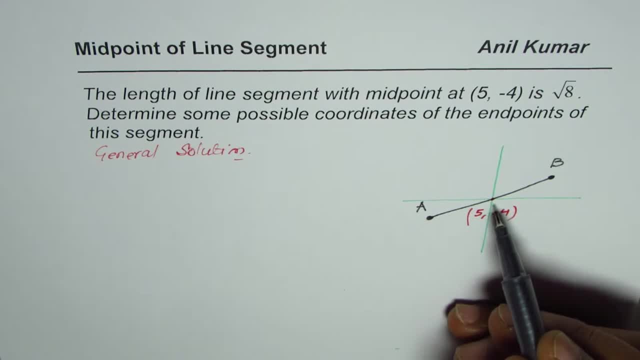 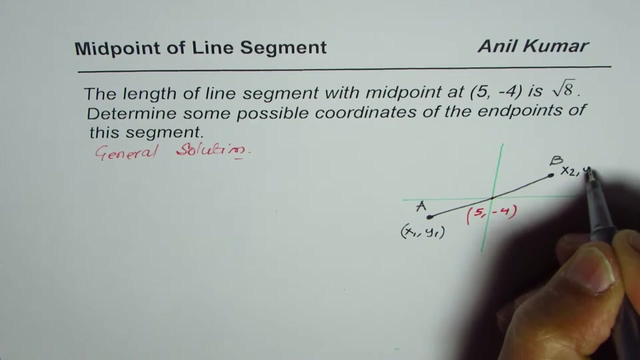 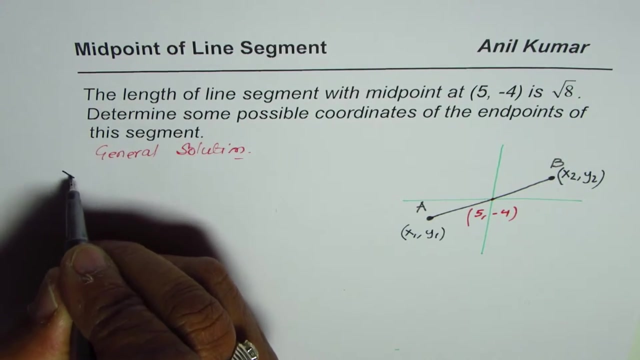 So let us say this line, segment AB, has midpoint 5 minus 4.. We need to find coordinates of point A and B, which are the endpoints, right? So let me write these coordinates as x1, y1 and x2, y2.. Since 5 is the midpoint, we can write our equation as x1 plus x2 divided by 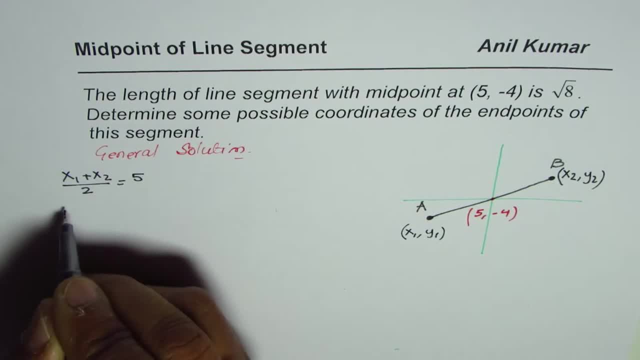 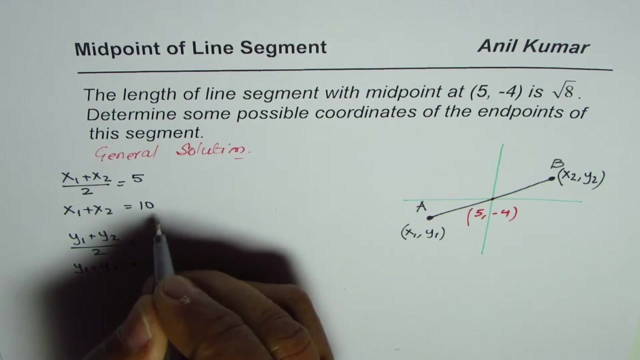 2 is equal to 5. That gives us x1 plus x2 is equal to 10.. We can get another equation by writing y1 plus y2 divided by 2 as equal to minus 4, or y1 plus y2 is equal to minus 8.. So we get two. 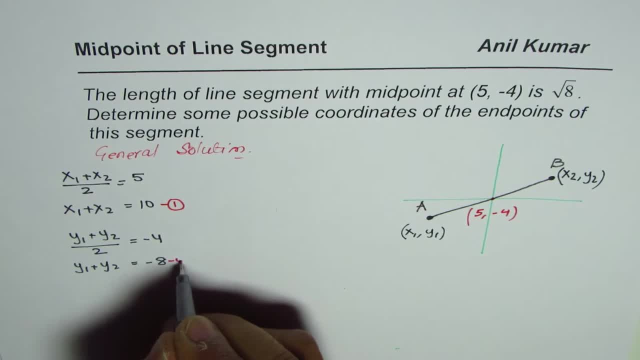 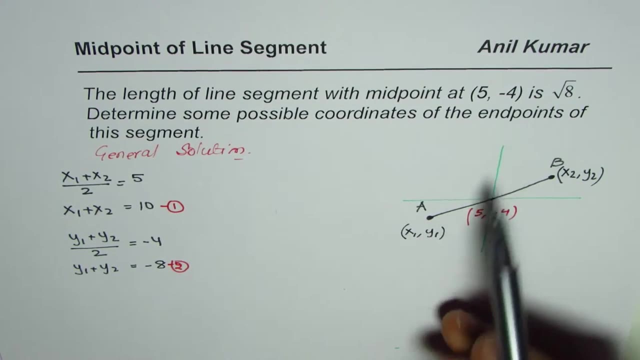 different equations, but we have four variables, correct, We have four variables. So indeed, we need four equations to solve this particular equation. We can get the other two by using distance formula, Since the distance between A and B is square root 8, distance formula. 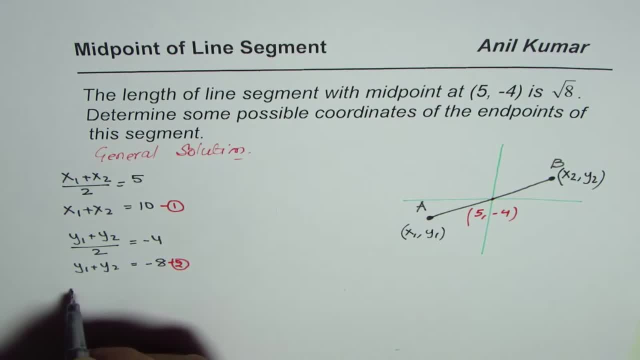 you know, is distance square, which is, let us say, d square, is equal to x2 minus x1 whole square Right, y, 2 minus y, 1 whole square right. In our case, distance square is given to us as square root of 8.. So we could write this as square root of 8 square, which is 8 right, and that is equal. 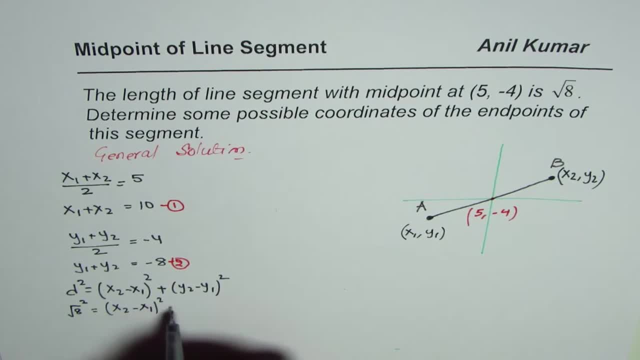 to x 2 minus x 1 square, plus y 2 minus y 1 square. So that is how we get one complicated equation. Now how to get two equations from here, that is the key for solving such equations. What we get here is basically: 8 is equals to sum of squares of two numbers To make. 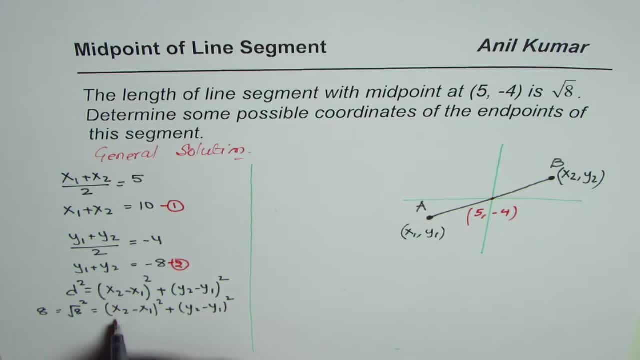 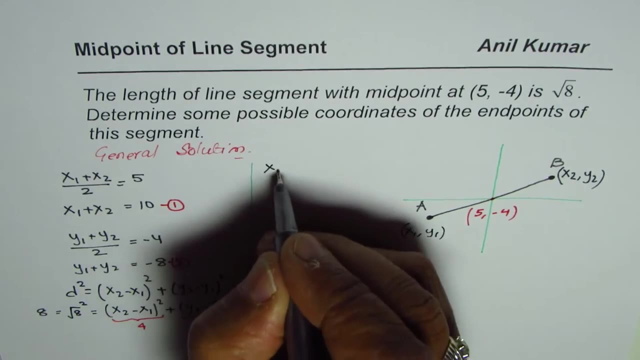 our solution simpler. we can say that this square is 4 and this square is also 4.. We know 4 plus 4 is 8, right? So what we are trying to say here is: let the equation be x2 minus x1 square. 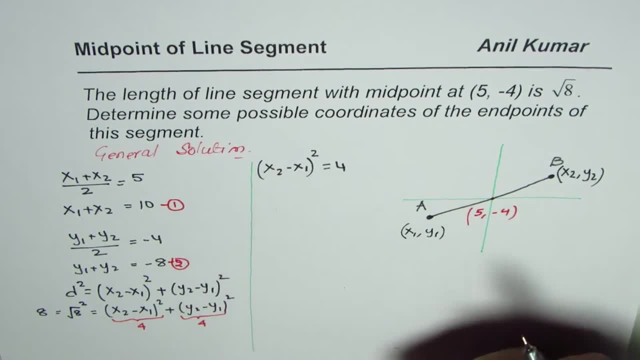 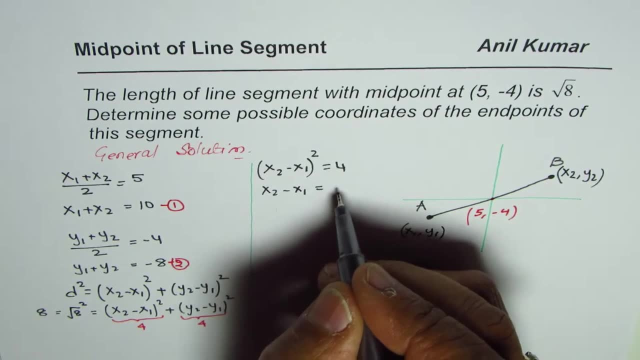 equals to 4, right, That means x2 minus x1 could be equals to square root of 4,, which is plus minus 2.. So when you do square root of 4, I mean let me write square root of 4 first. 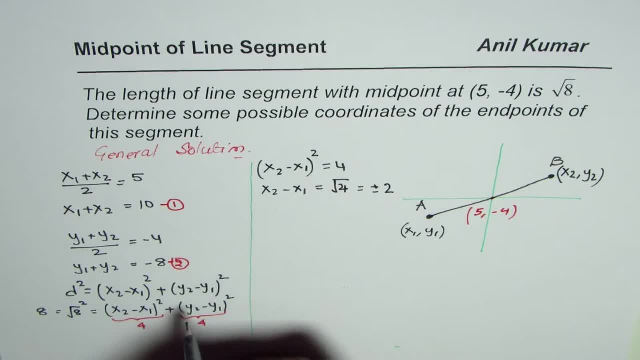 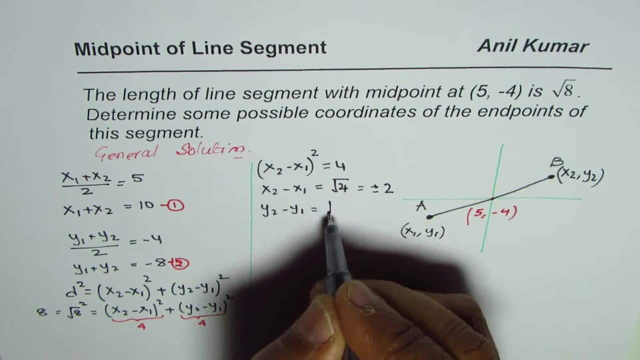 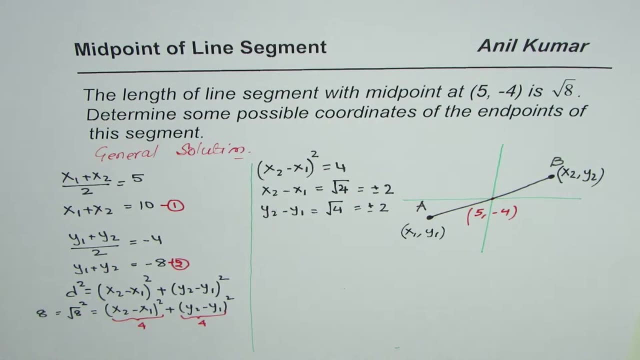 which could be plus or minus 2.. So we get two equations from here. Similarly, we can say: y2 minus y1 is equal to square root of 4, right, Which could be plus or minus. So that gives us two more equations. So we do have now four equations to solve. 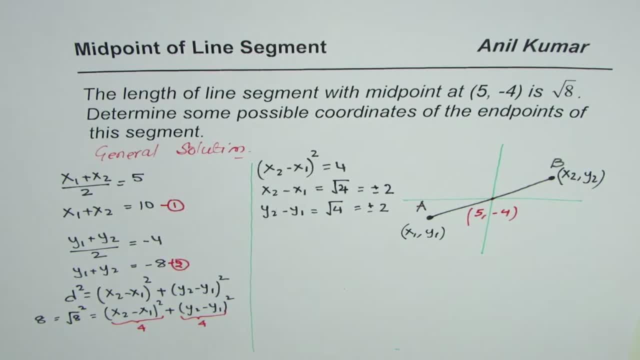 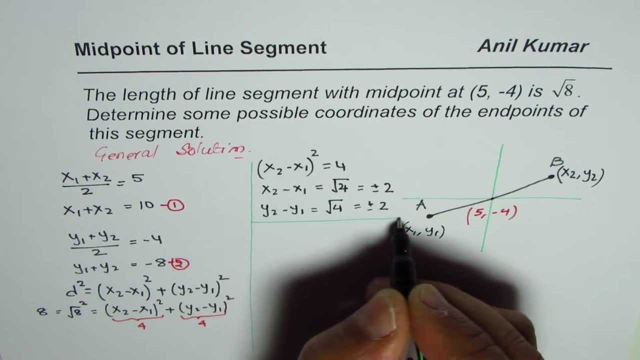 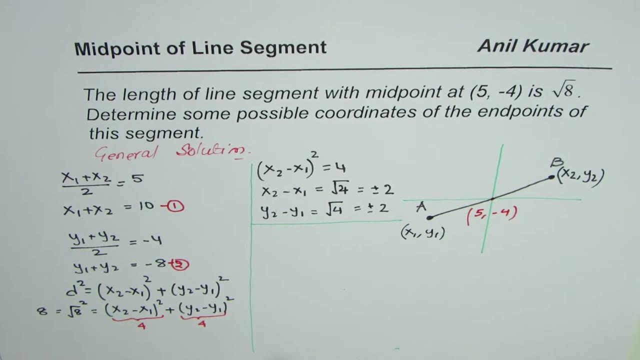 and get the values of x1, y1, x2, y2, right. So now I hope you appreciate how to solve such a question. You can actually pause the video at this stage and find the solution right. So what we will do here is continue with the solution. 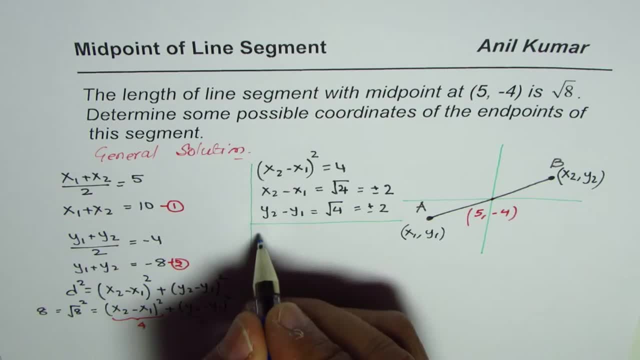 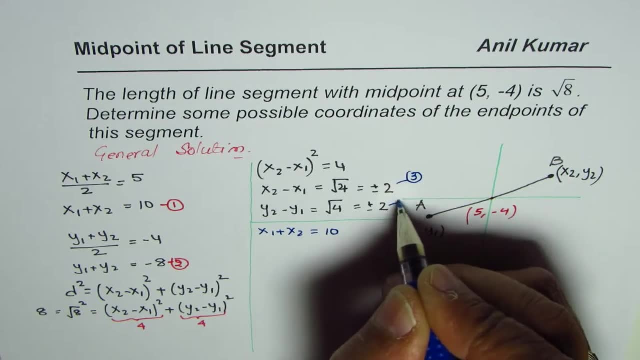 Here is how We will continue. So we have equation 1 as x1 plus x2 equals to 10.. We will call one of these equations as 3,, the other one as 4, and we will select positive numbers, just to make it simple. 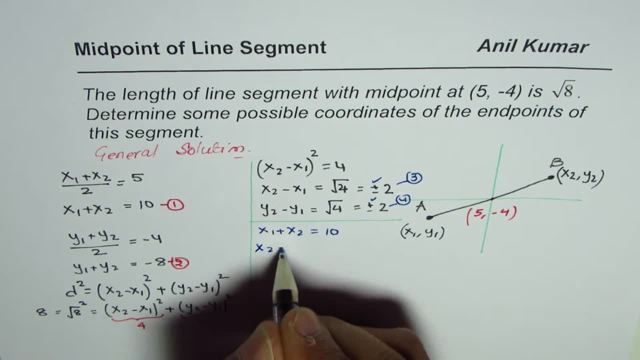 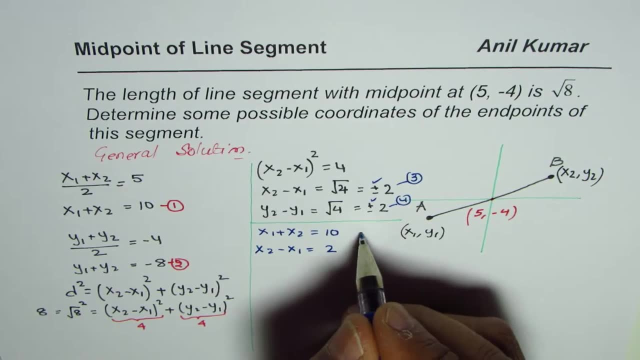 right, So we have x2 minus x1 as 2, right So these two equations- that is from equation this is our equation 1, this is equation 3.. Now, if you add that equation, you will get x2 minus x1, square root of 4, right So? 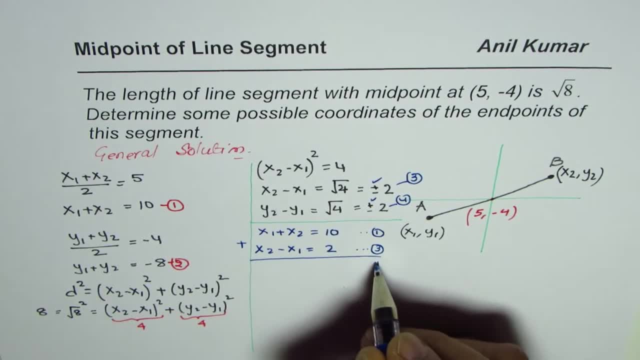 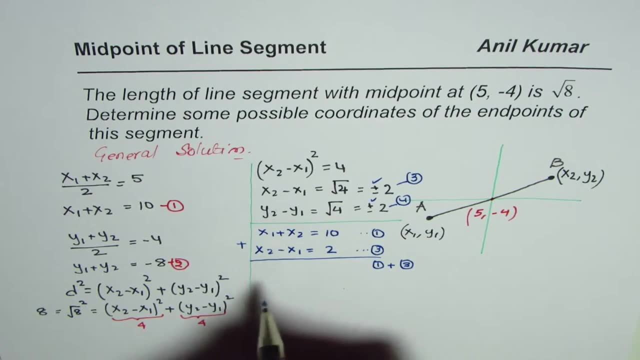 if you add them up, right, If you add these equations, that is to say, if you do equation 1 plus equation 3, then what do you get? x1 minus x1 is 0. You get 2 times x2 as equals. 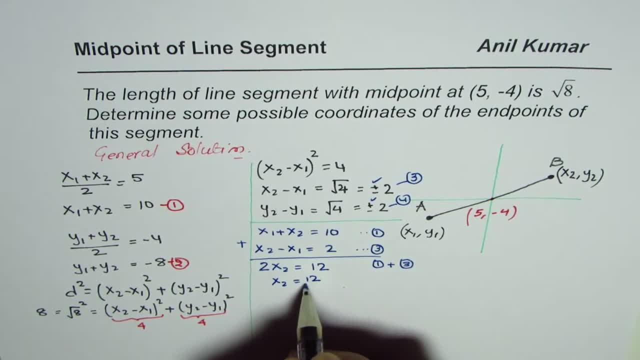 to 12, and then x2 is equals to 12 divided by 2, which is 6.. So you get the value of x2.. Once you get the value of x2, you can find x1, right? So from equation 1, we know. 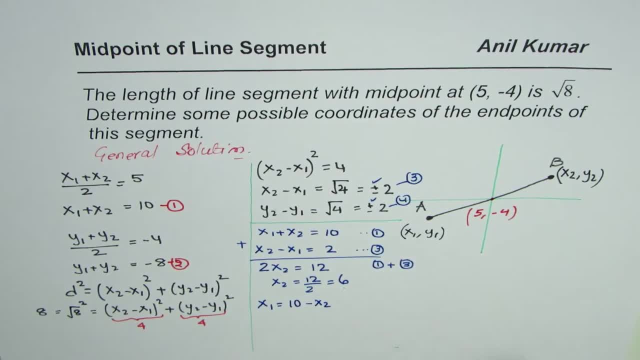 x1 is 10.. So we have x1 minus x2 as 2, right? So from equation 1, we know x1 is 10.. So we have x1 minus x2 as 2, which is 10 minus x2,, which is 10 minus 6, and that is 4.. So 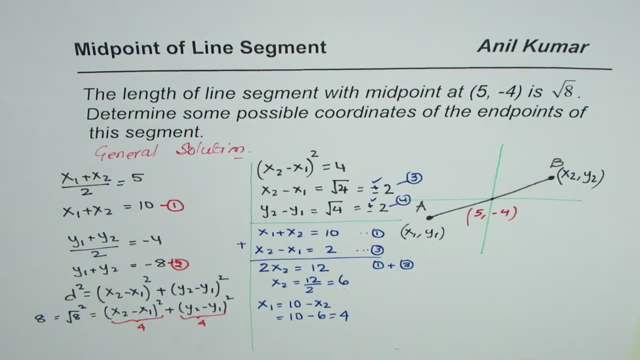 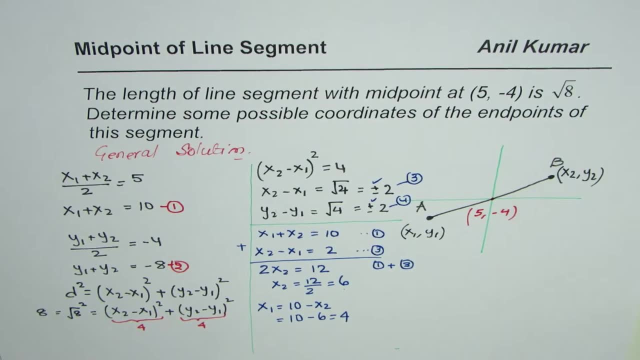 we get the value of x1.. You get an idea. right, So we get values of x1 and x2, right? So we got the x coordinates for both the points. Now let us find the y coordinates. So, strategy. 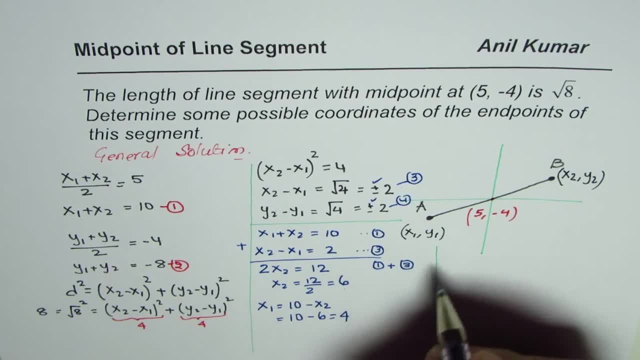 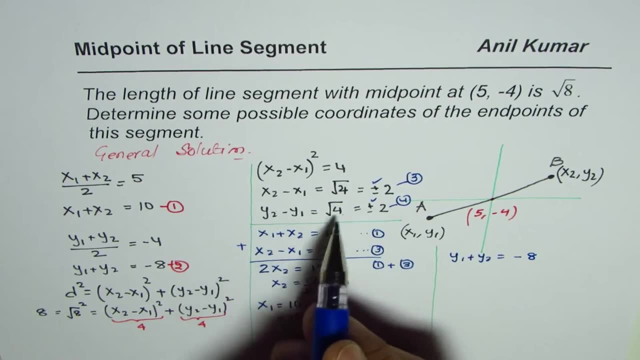 is exactly the same. We do have one equation, which is: y1 plus y2 is equal to x1 plus y2.. Now, from here, two equations we could select. we will select with positive 2. So we could. 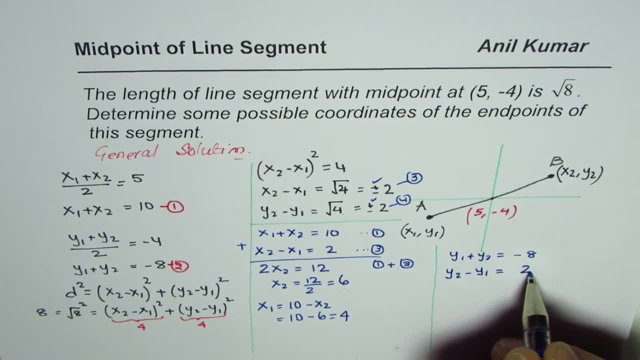 do y2 minus y1 as 2, right Now, when you add this, let me call this: this is our equation number 2, and this is equation number 4.. So, if you add equation 2 and 4, if you add them, 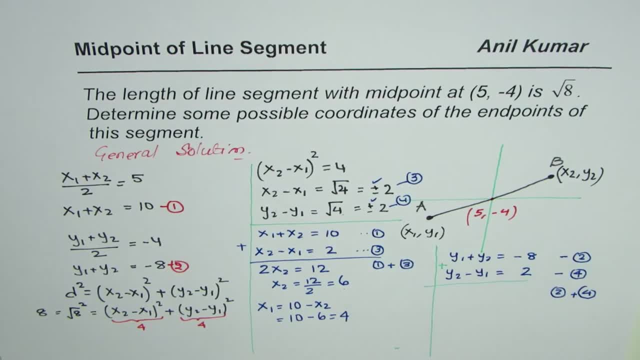 up right. So what we are doing is kind of adding them up right. So if you add them, y1 minus y1 is 0. So if you add them, you get y1 minus y1 is 0. So if you add them, 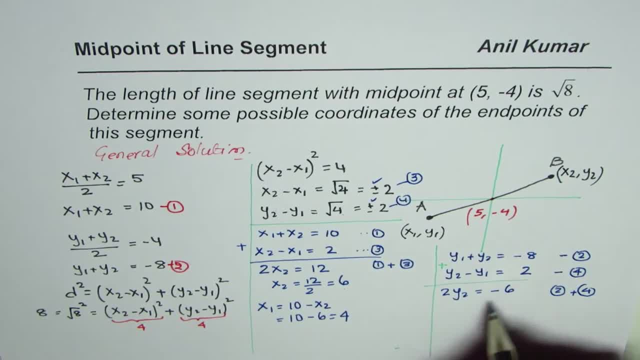 you get: 2y2 equals to minus 6.. y2 is minus 6 divided by 2 as minus 3.. So we get y2.. You can find y1 using one of these equations: y1 is equal to minus 8, minus y2, which is: 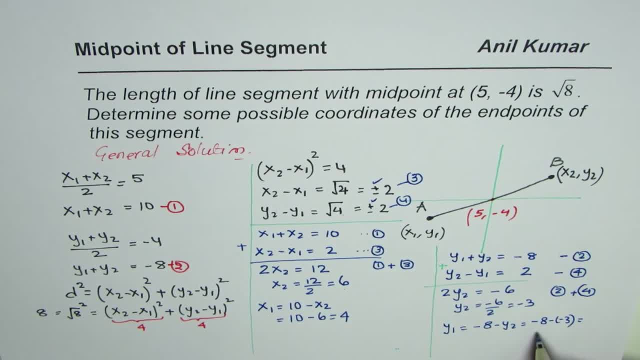 minus 8, minus minus 3.. So which is minus 8 plus 3 or minus 5, right? So we get the 2s as minus 5.. So we have these values with us right Now. once we have the value, we 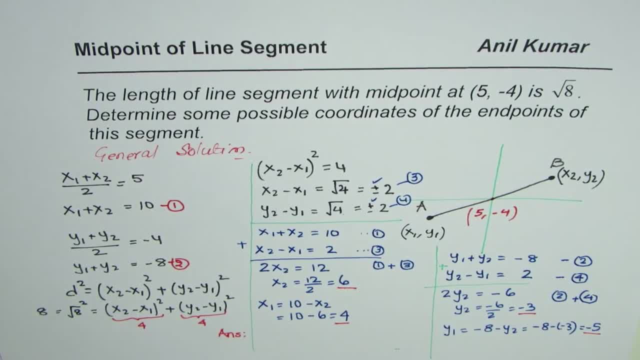 can write down the answer. So the answer for us is the coordinates for point A, which is x1, y1.. x1 is 4. y1 is minus 8. And x2, coordinates for point B. let me write B here. 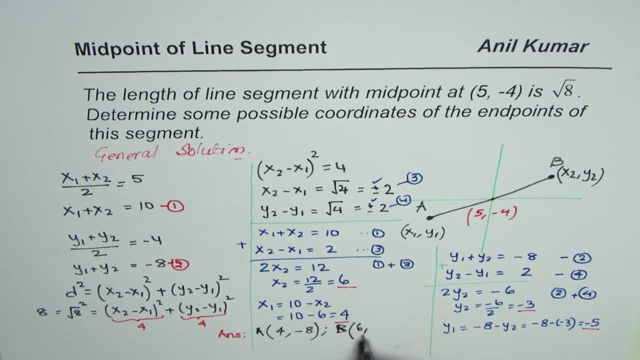 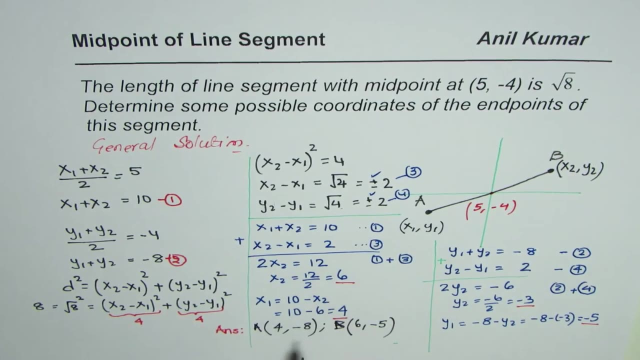 you know, B is x2, y2,, which is 6.. And y2 is minus 5, right, So 6 and minus 5.. You can check if the midpoint is 5 and minus 4 or not. Add 4 and 6,. 10, divided by 2 is 5.. Add minus 8 and minus 5.. 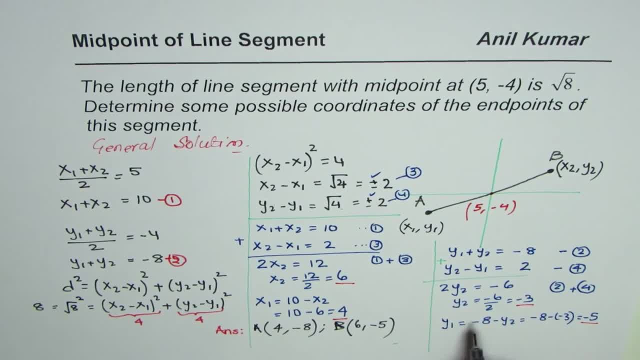 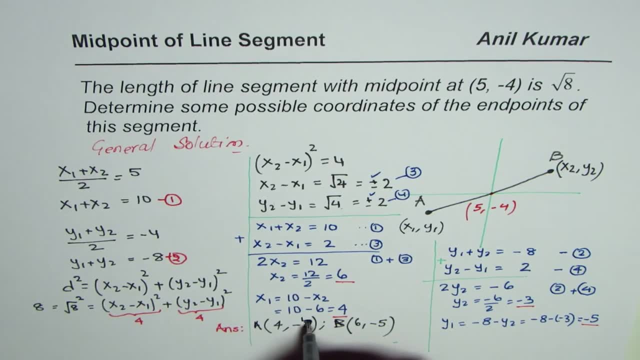 So there is a mistake here. Sorry, y1,. as you can see here, y1 is minus 5.. I wrote it wrong, So y1 is minus 5.. I'm sorry. And y2 is minus 3.. So this is minus 3.. So that. 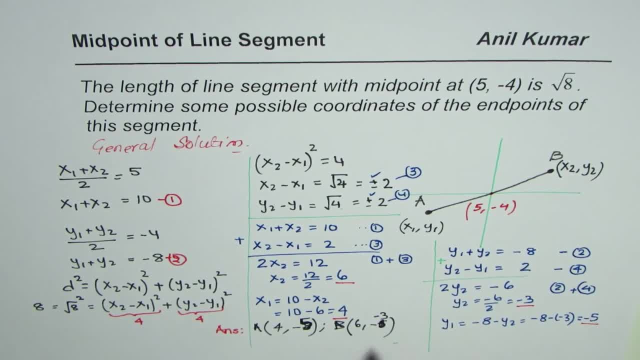 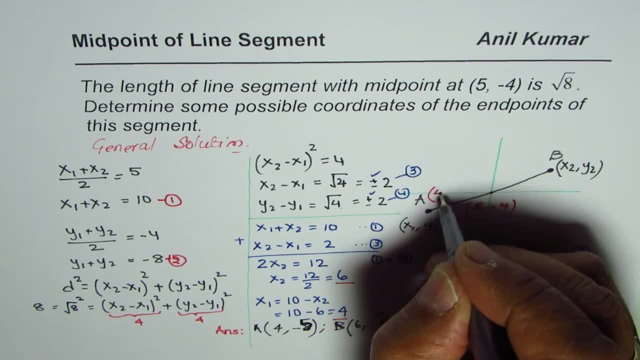 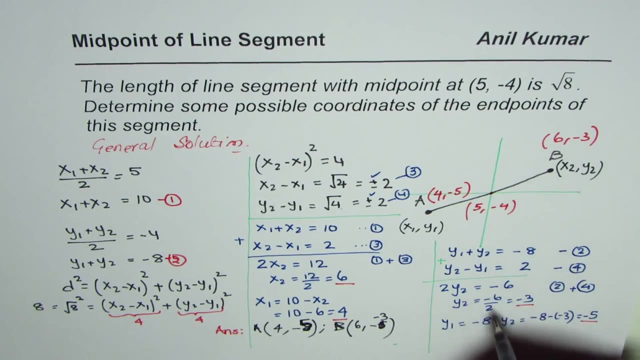 is y2, right. So that is the solution. So let me write down clearly the answer. right? So we get coordinates for point A as 4 minus 5 and coordinates of B is 6 minus 3, right. 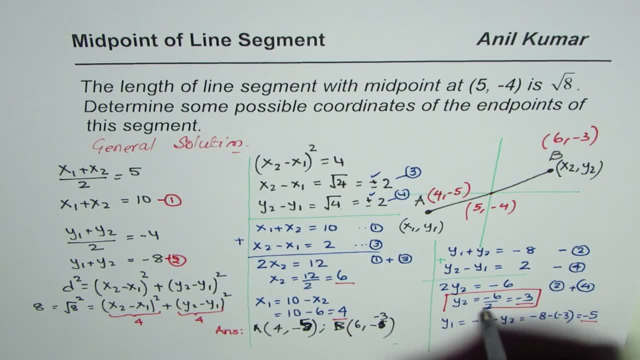 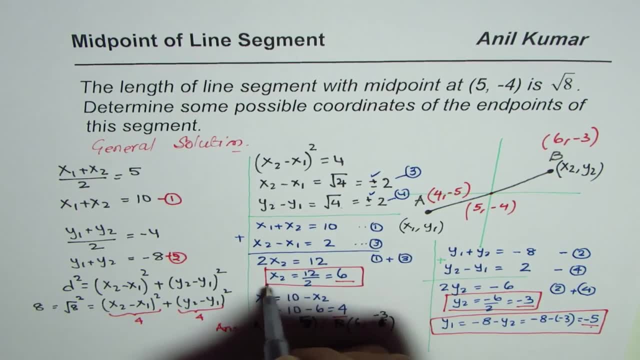 So that is your y2, right, This is y2.. This is y1, minus 5.. Correct, And x2 is 6.. x1, we say x1 is 4, right, So this is x1.. 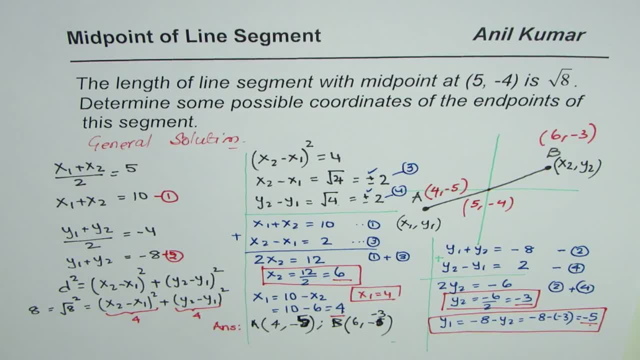 So that is how you solve this particular question. I hope the strategy is absolutely clear. Thank you and all the best.